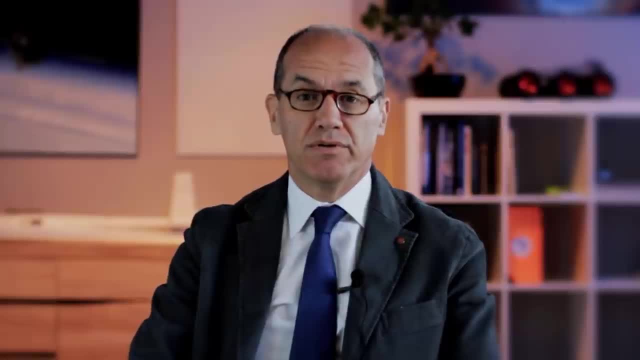 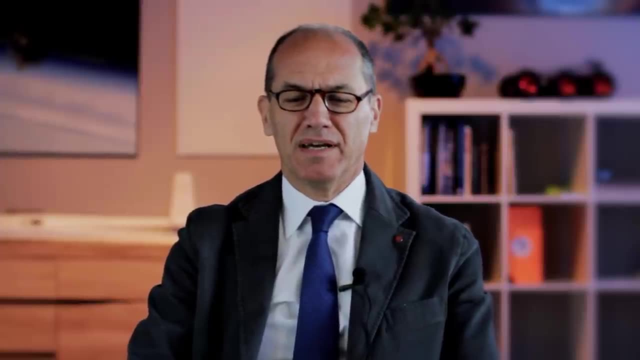 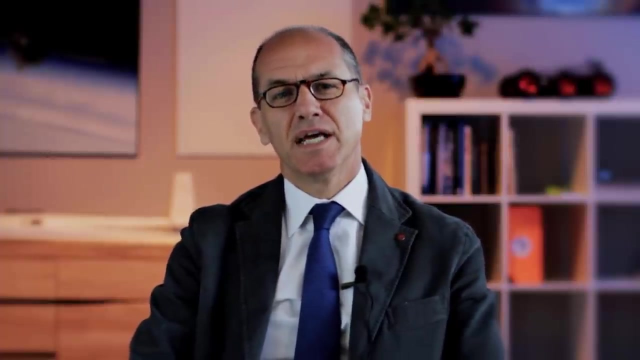 I am the coordinator of the PhD course in aeronautical and space engineering. My background in research starts from structures. I practiced a lot computational mechanics, finite element techniques, Then I moved to composite materials, composite structures and recently I entered the field of smart structures technology. while being interested 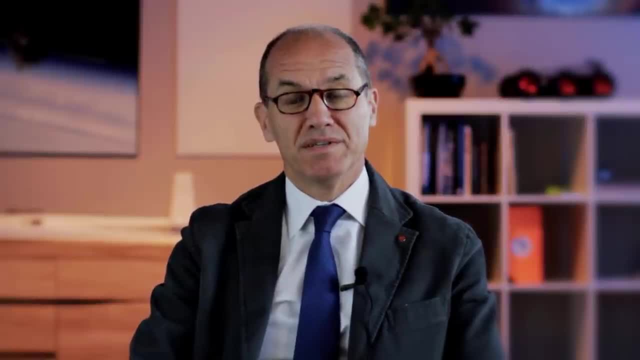 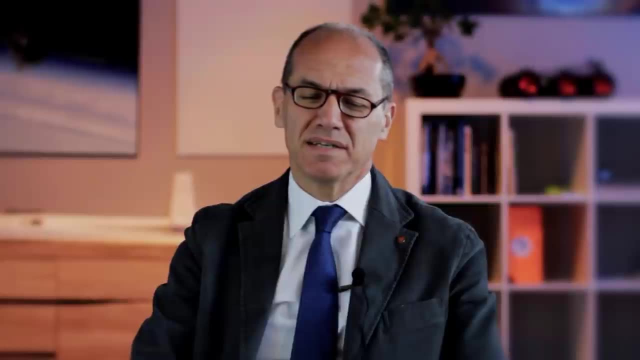 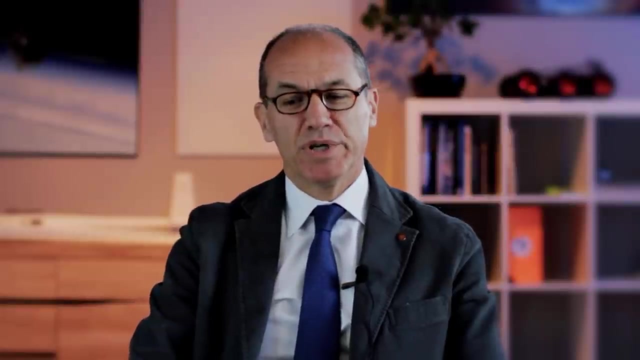 in all those years in space systems and satellite systems as well. So my involvement in satellite system lasts since 15 years and during all those years I've been working in the space systems and satellite systems as well. I've been working in the frame of our professional 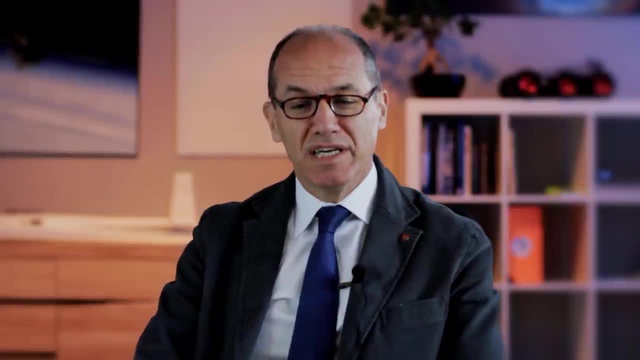 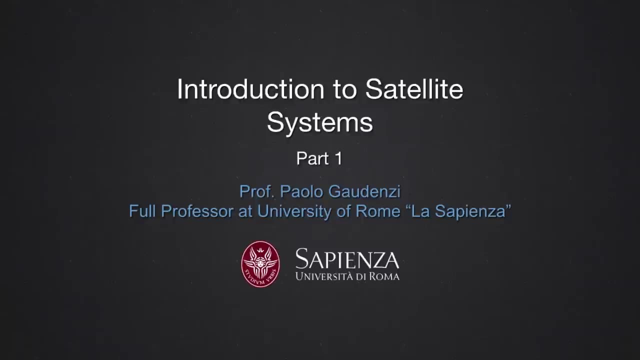 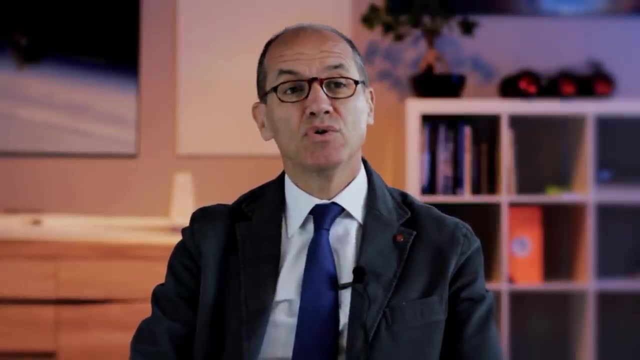 master in satellites at La Sapienza, and today I'd like to make you a short introduction on satellite systems. My agenda for this talk is first considering a system view on space missions and all the engineering challenges that are related to the mission. Then I will. 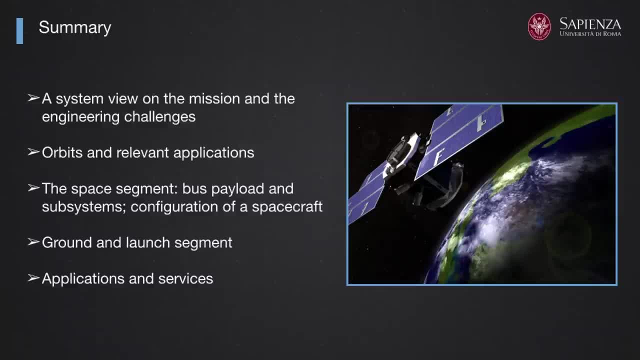 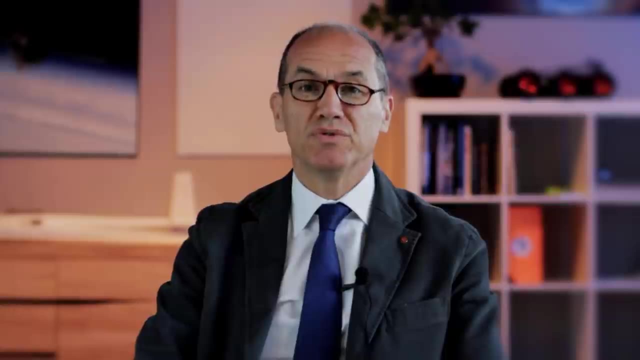 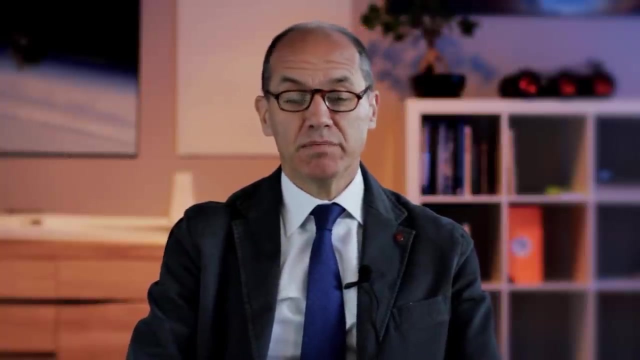 shortly move to orbits and all the applications that we have for our satellite systems, First for each orbit around Earth and also for all the trajectories that the space system might have leaving the Earth orbit and moving to space systems in the solar system and even beyond it. Then we will touch a little bit the space segment to see how a spacecraft 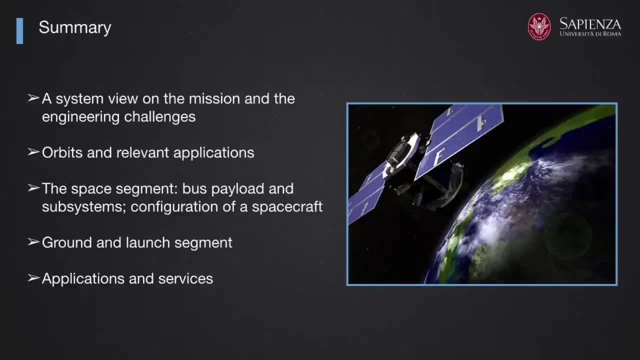 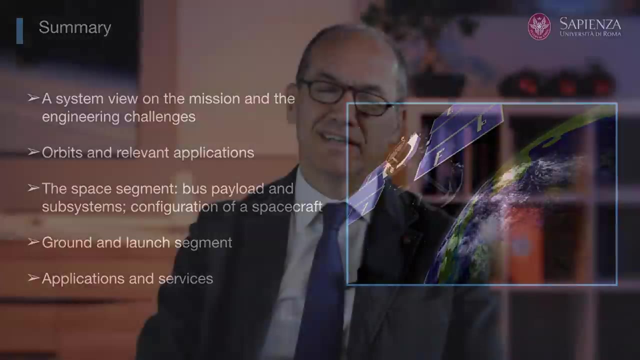 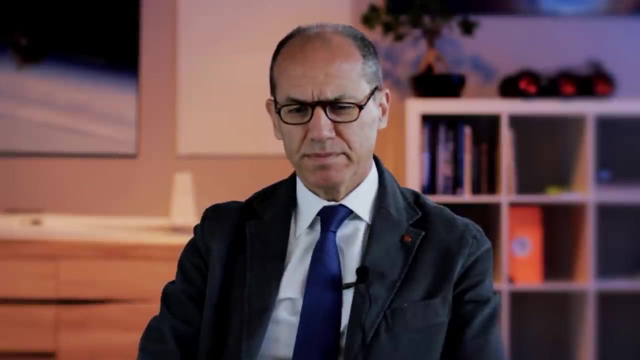 is composed by vast payload and subsystems, and we will enter a little bit the configuration of a spacecraft. We will briefly touch ground and launch segment and then we will be discussing a little bit about applications and services, not only of space activities of today, but also a little bit of space activity of tomorrow. So let us start with talking a little bit. 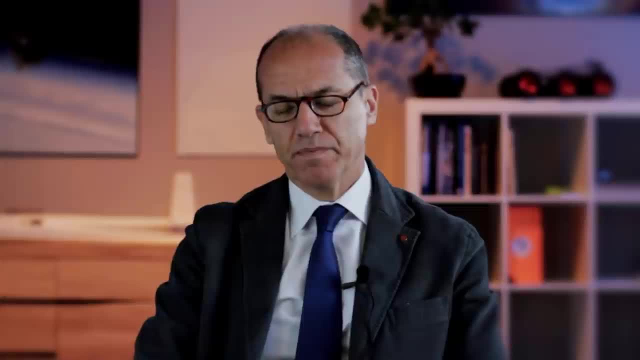 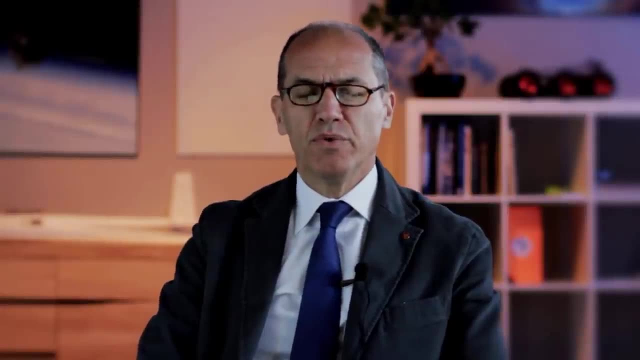 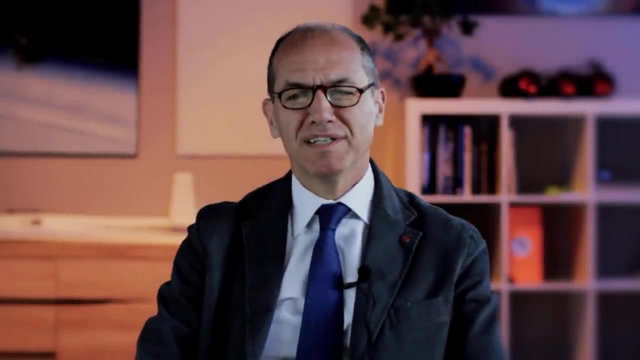 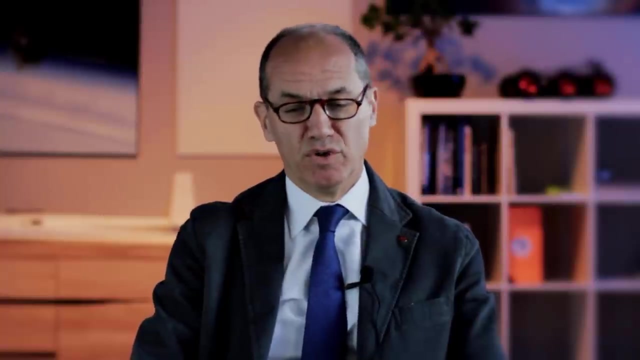 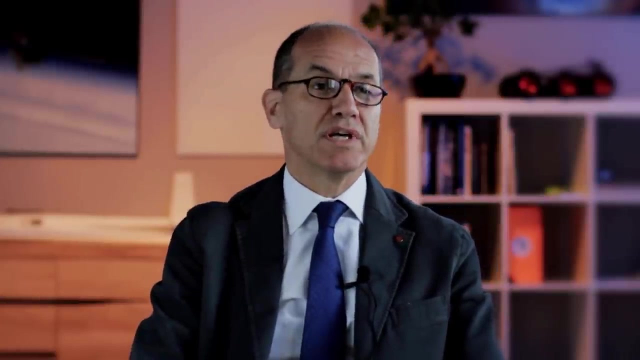 about space missions and space systems. So performing a space mission Is a real challenge. It's very difficult to reach an orbital position, very hard to leave our ground and to be stronger than the force of gravity, leaving our level and reaching the level of an orbital position. So to go to space we need first of all a launch segment. 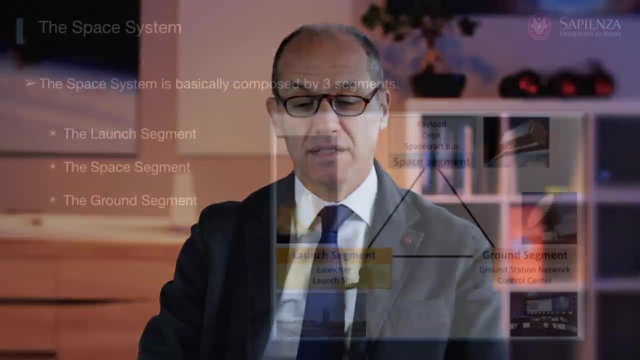 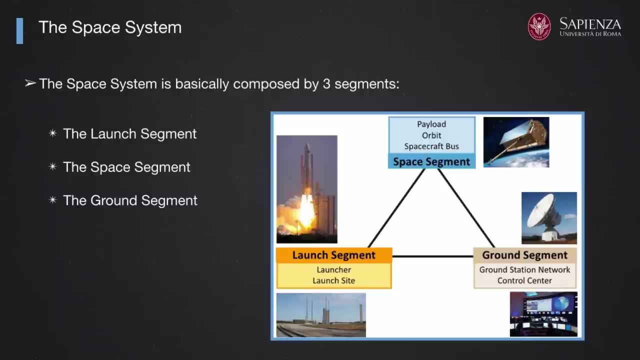 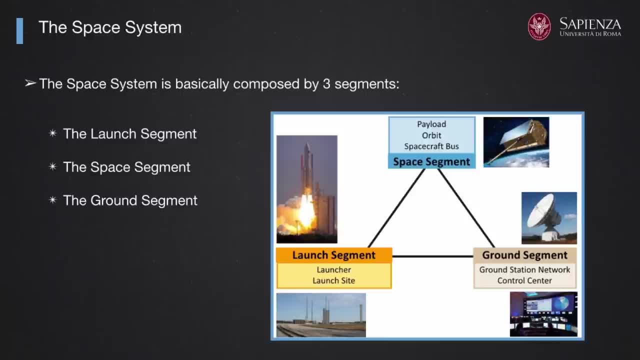 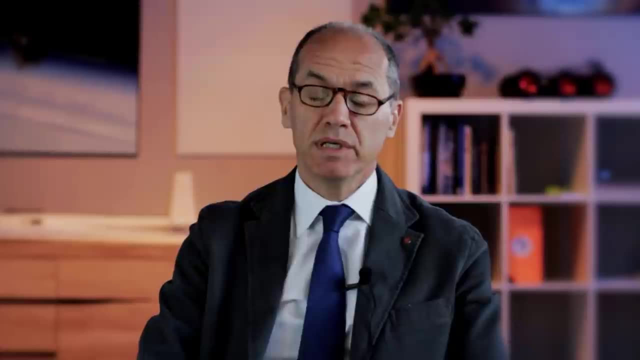 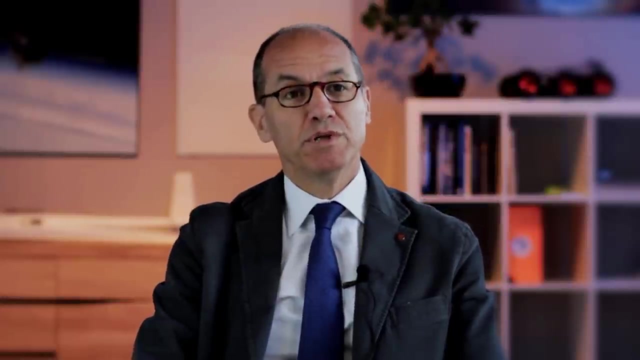 of our mission. While on orbit, the satellite will perform its mission and will get in contact with us on ground by means of the ground segment, from which all the signals coming from the satellite will be received and the mission of the satellite will be finalized. So to perform a space mission, you need a system that is composed by three segments: the launch. 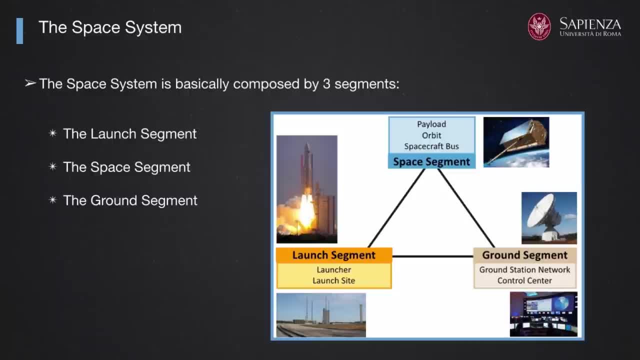 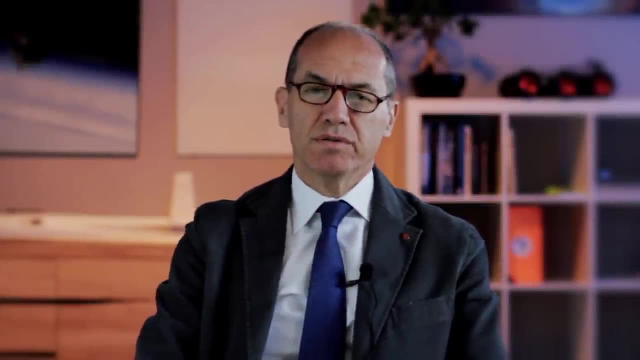 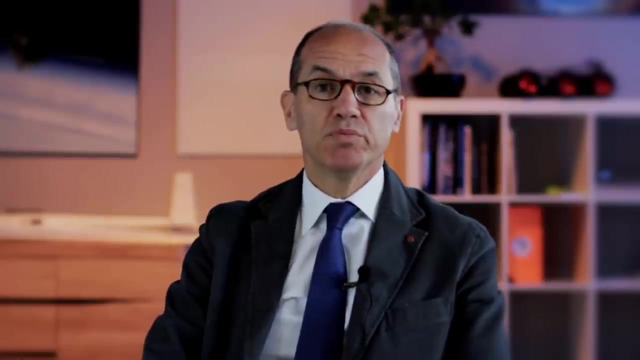 segment, the space segment and the ground segment as well. So a rather complicated organization of things and phases and parts and there are a lot of engineering challenges because space environment is very hostile, Not only difficult to be reached but very hard because there is no protection from the atmosphere. 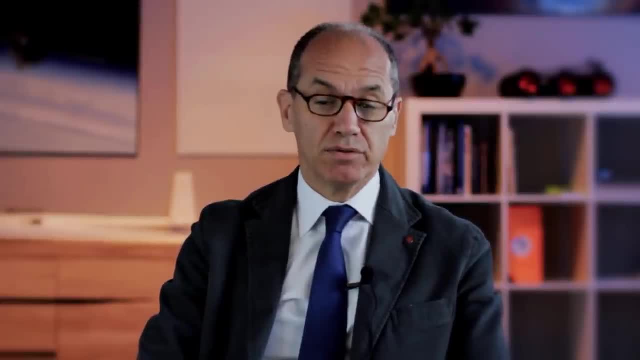 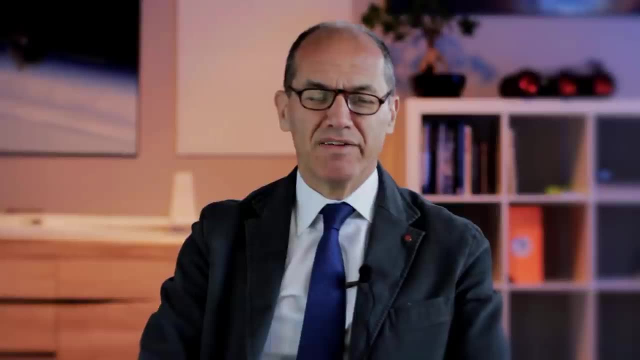 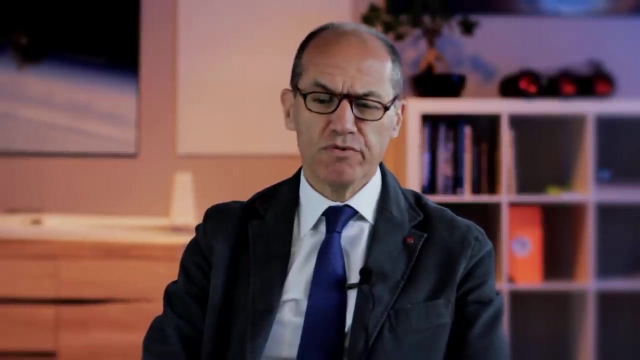 So the rays from the sun are coming directly to the satellite and in this empty space you have no way of having an easy access to energy. So you have to capture the energy by the sun to provide the energy for your satellite. In the empty space, the satellite has to point Earth in order to 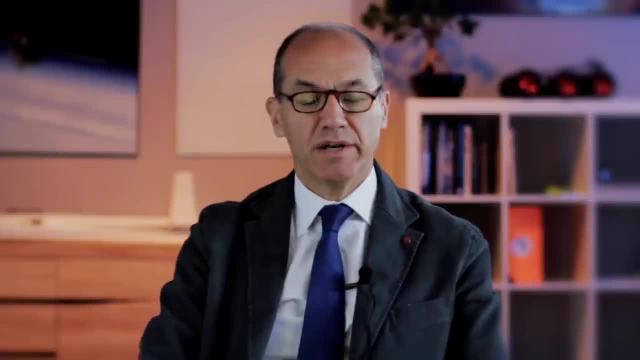 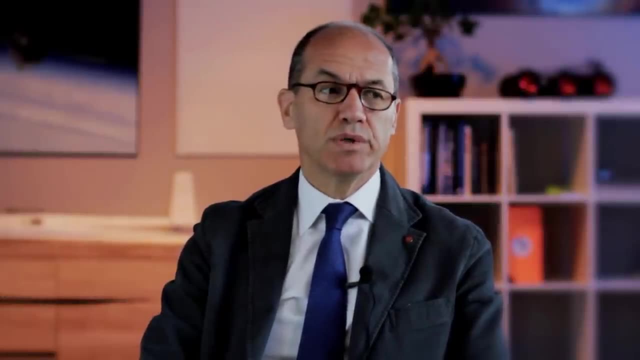 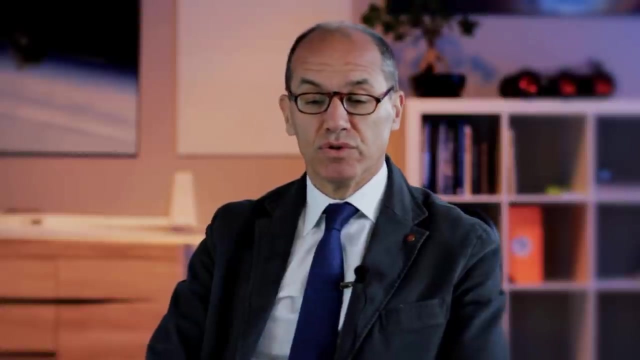 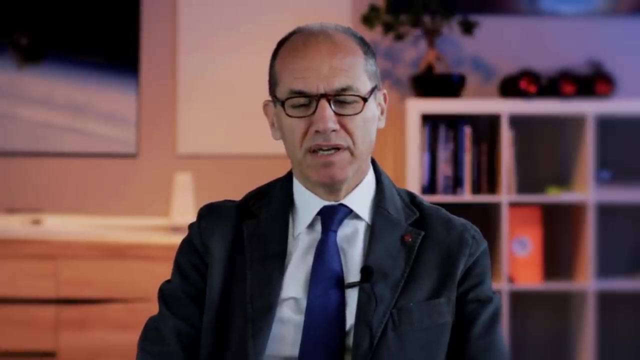 have the correct direction for the antenna and point the ground segment. and you know you need also to communicate with your ground segment all the data that you are capturing with your sensors, and also to inform your ground-based systems on how the system is performing, on how the satellite is. 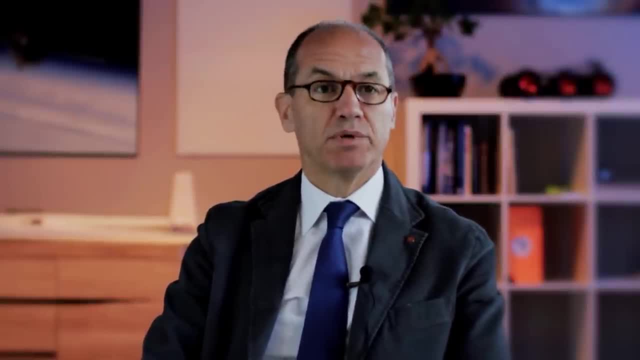 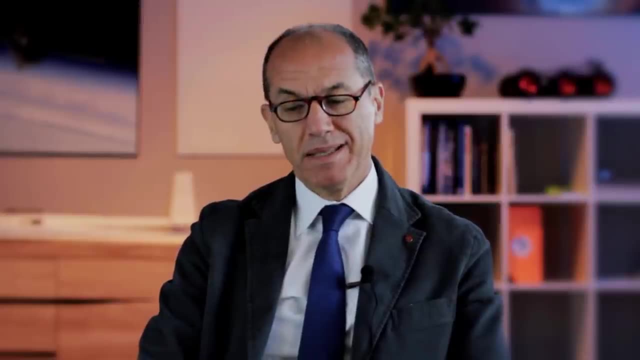 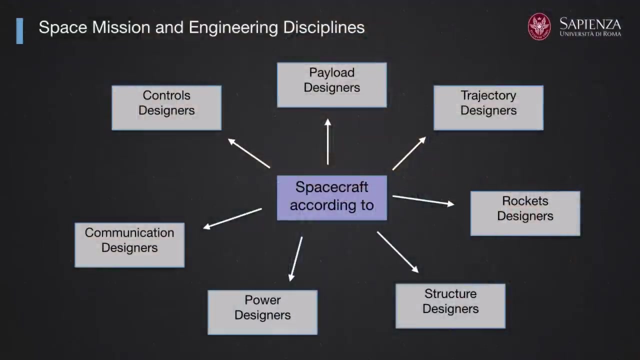 working, if it is working properly or not, Or if there are some problems. So a really complicated system. But there are a lot of engineering, sciences and disciplines that are needed to perform such a mission. First of all, you need to know. 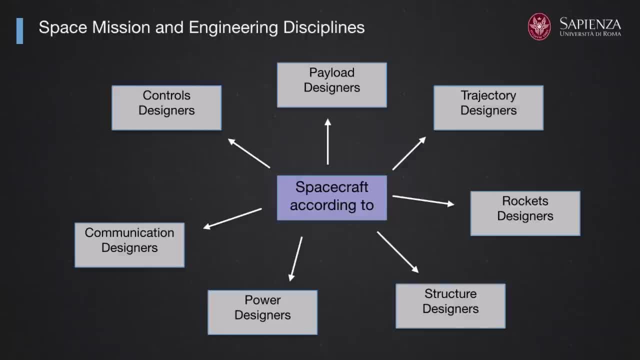 about flight mechanics, astrodynamics, meaning the trajectories that our system should perform in order to perform its mission. Then, of course, before that, you need to do some rocket science in order to have your missile, your launcher, to project our satellites in the right orbit. Then you need some electrical engineering to 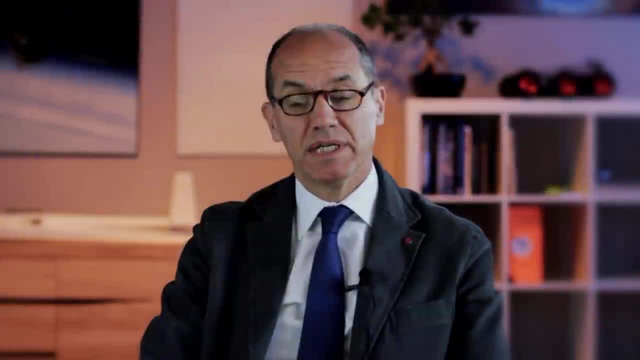 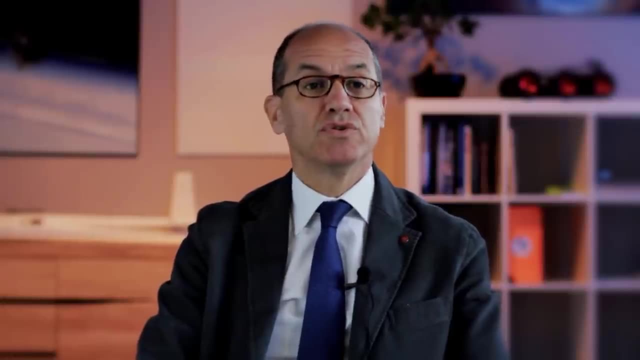 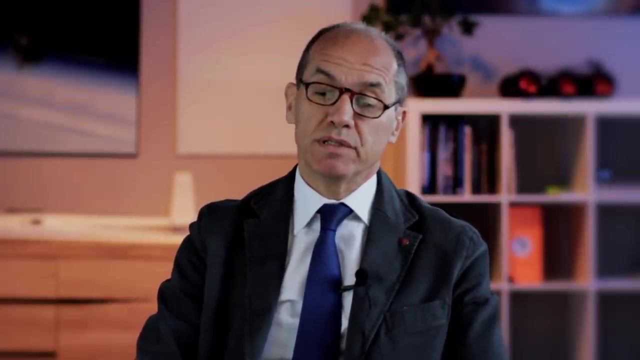 provide the power that you need by means of the solar panels that will collect the energy from the sun and transform it in energy that could be used first of all for for the payload of our satellite, that is to say, the ensemble of instruments that really provide the functionality to the mission, For instance, in a 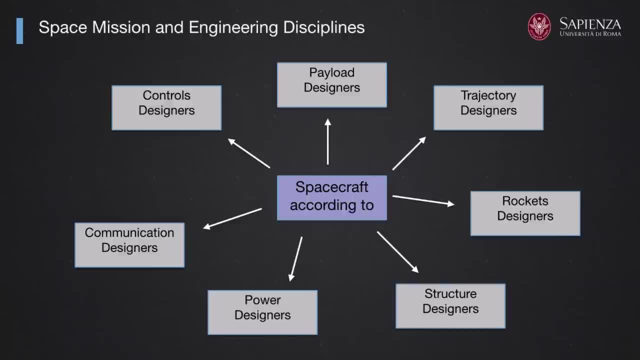 telecommunications satellite. the payload will gather the signal from Earth stations and project all the information in the area that is covered by satellite, meaning, for instance, that we are watching our space TV channel and the satellite is providing us either a movie or a football match by means of the. 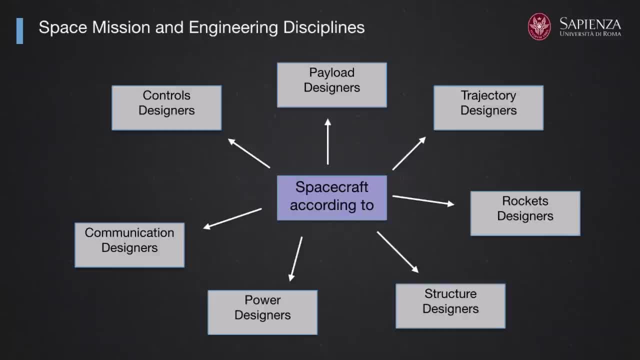 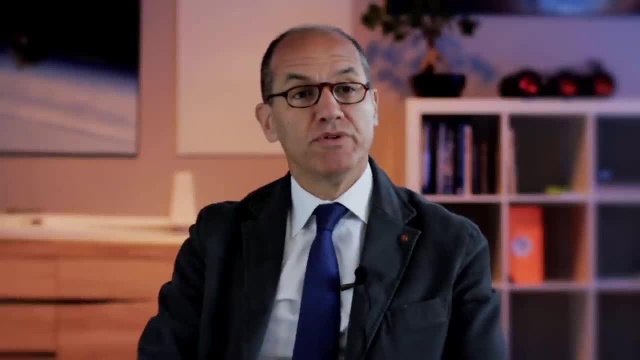 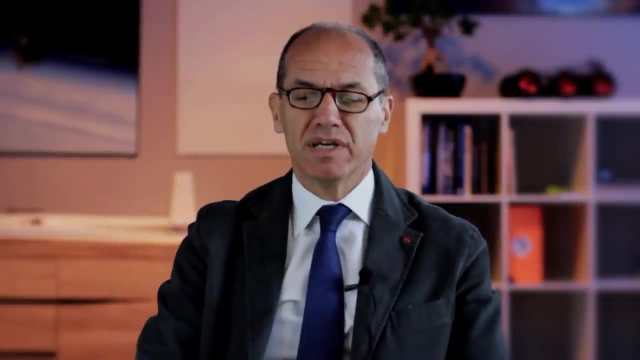 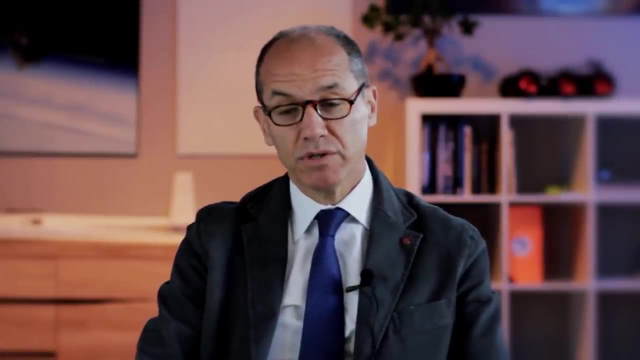 payload that is mounted on board the satellite, And this payload needs, of course, energy to transmit such signal, As I mentioned before, the satellite needs also to have a good pointing system. So there is a lot of engineering science behind the attitude, control system and trajectory. 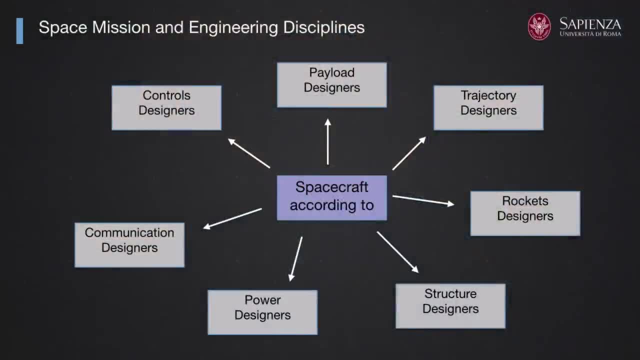 control, to assure that the position of the satellite is the proper one and the attitude, that is to say the position in terms of angular pointing with respect to Earth, is in the proper dimension, in the proper situation. So, in order to perform a space, 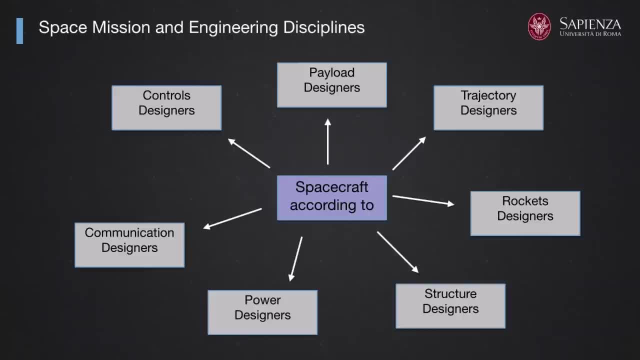 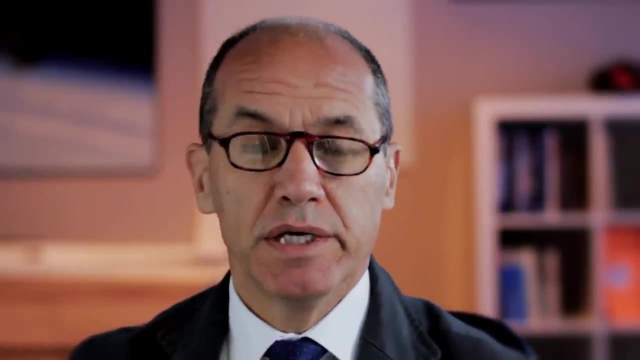 mission and to construct a space system, you need a lot of competences, you need a lot of expertise that needs to be combined together for the functionality of all the parts of the spacecraft, of the launching system and of the ground segment as well. 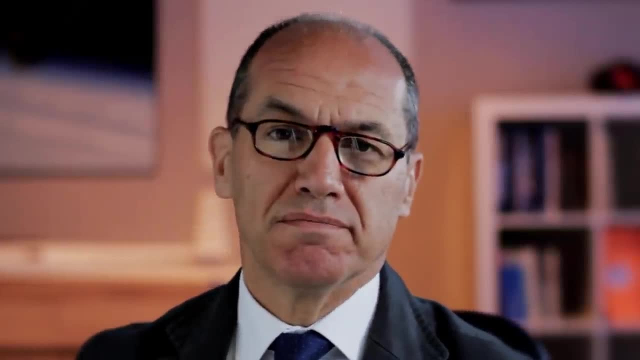 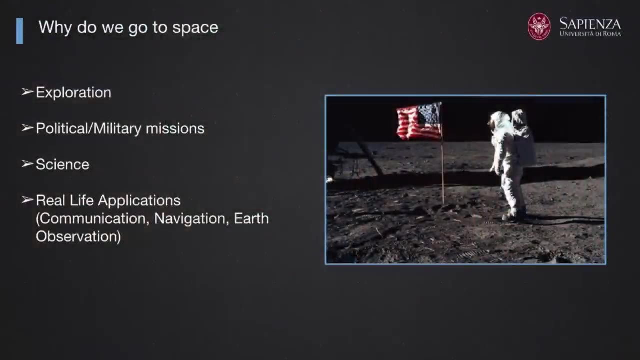 But why going to space? What are the reasons for performing a space mission? Why going to space? What are the reasons for performing a space mission In the past and also nowadays? the first impulse to Go Space is to perform some exploration activity or 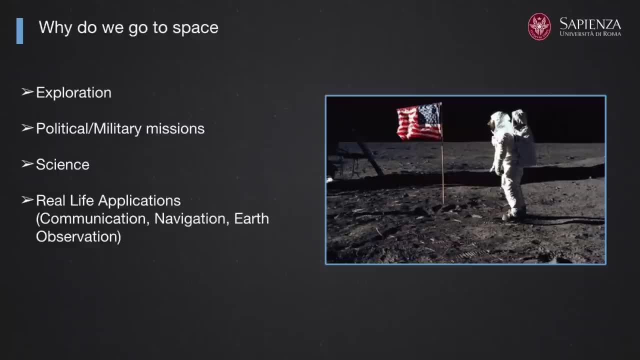 some science mission. This is maybe the first idea that is related to the tendency of mankind to go beyond limits, to go beyond our horizon and to see what's next. what's what's next, what's close and else part of our basis of scientific work systems. 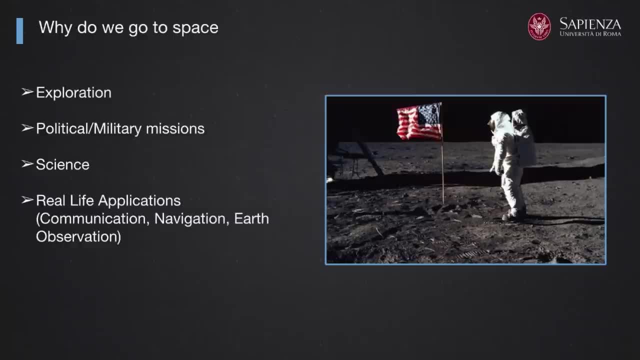 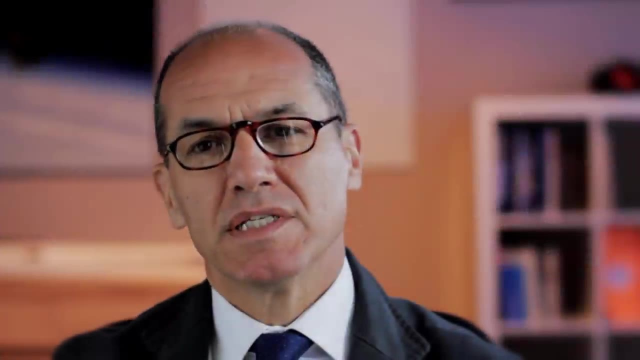 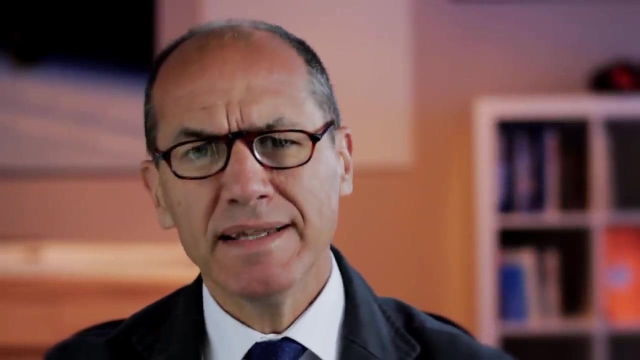 close to us, or even what's in space, what's in the world beyond our capability of looking, because beyond our capability of looking around. So exploration and science is the first reason why to go for a space mission in space. Then there are, of course, a lot of political or military reasons to go. 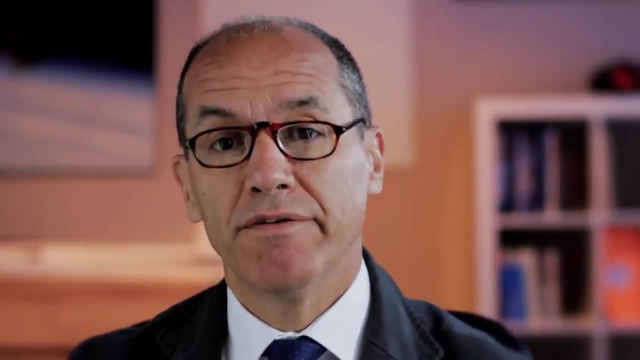 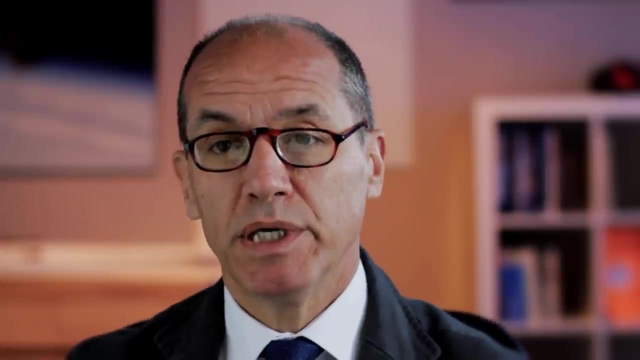 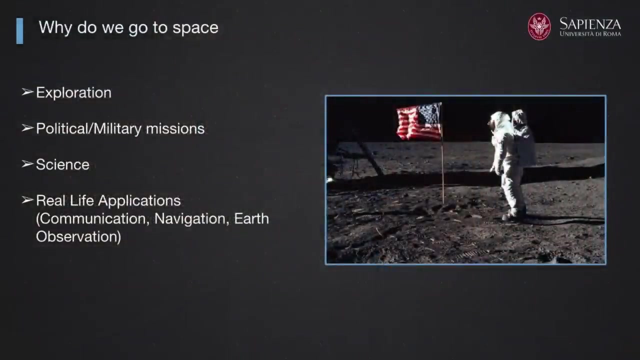 there because of course, from space you really have the idea of a global view on our planet, and global view might be geopolitical control or having some access to information from a global viewpoint, and of course there are a lot of military applications that could be of interest. But apart from 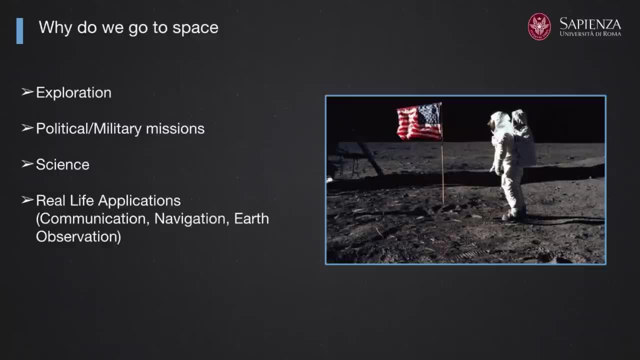 science. apart from political reasons, there are a lot of practical reasons for going to space. In fact, there are a lot of applications and services that are really useful for everybody, for the single citizen of our planet Earth, like the applications in Telecom. 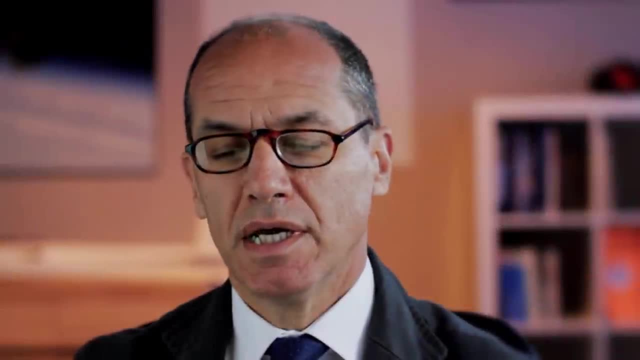 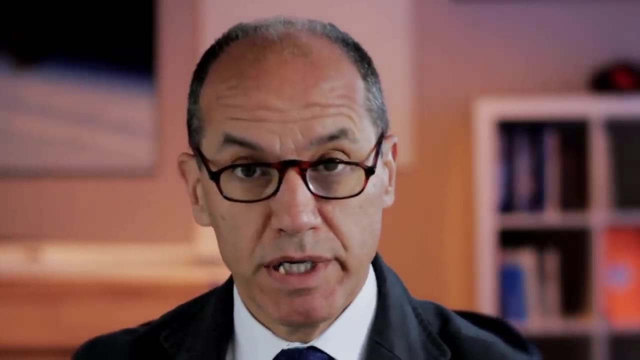 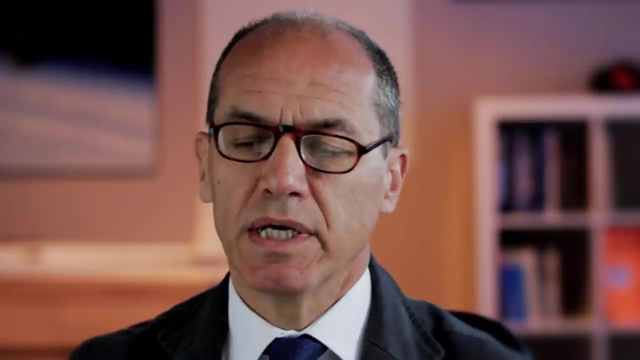 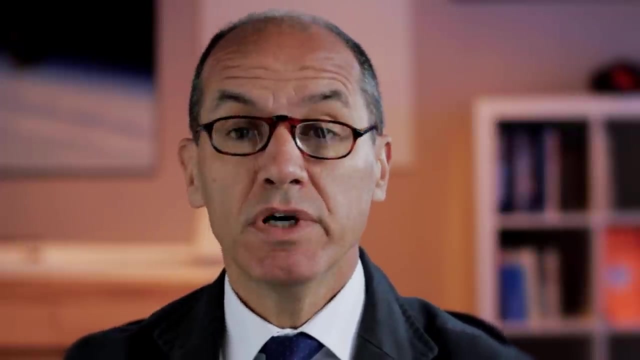 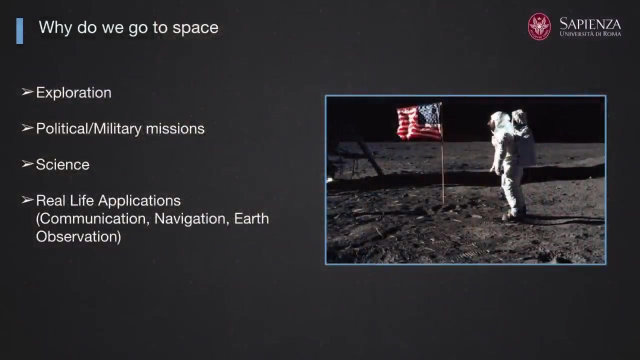 and everybody can experience how important is having services like space television or space-based television, But now we experience also the importance of having navigation and positioning systems that are based on satellite assets. Furthermore, by means of Earth observation capability, we can provide not only to the single citizen but also to organization, to governmental agencies. 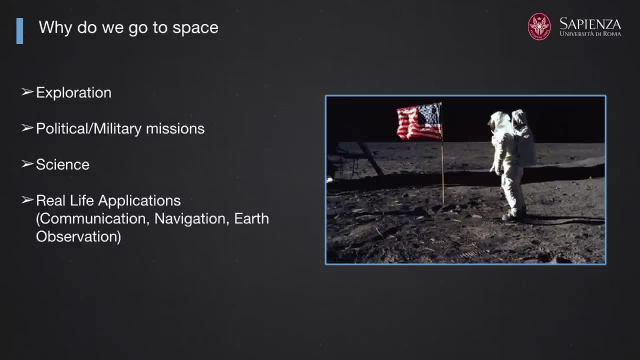 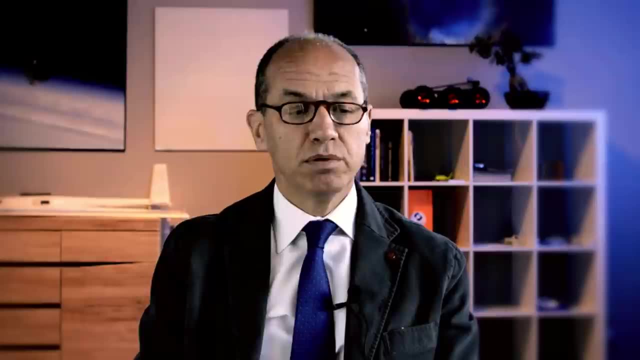 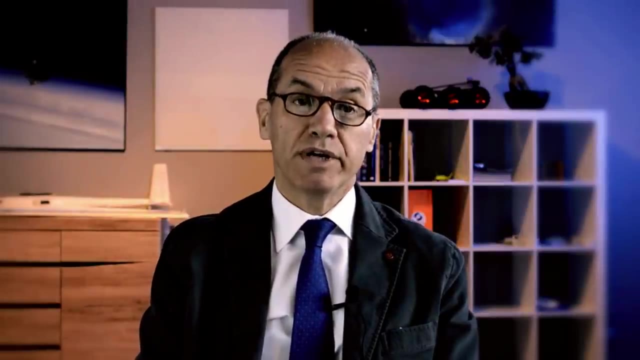 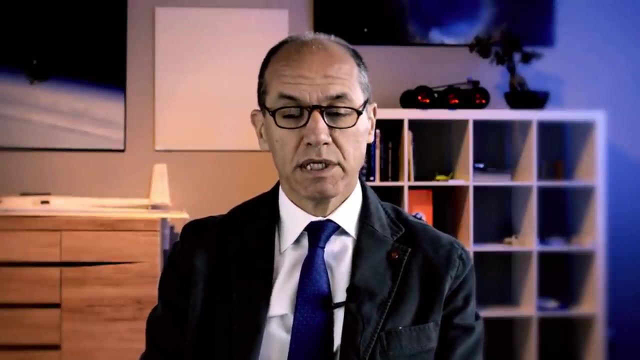 and to regional governments a lot of information on the use of ground, on the evolution of climate, on the possible use and misuse of our ground, and these are all applications that are very useful in practice. So space is important for science, for politics, but also for real-life application, for the benefit of everybody. 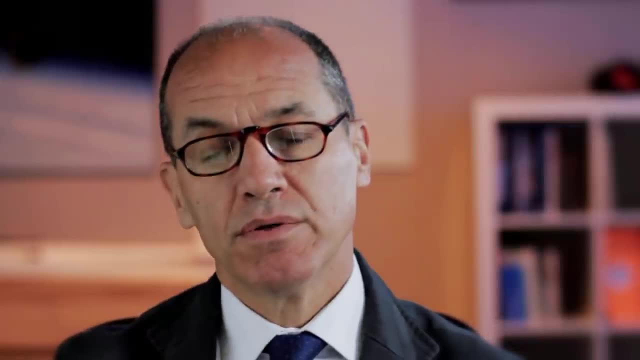 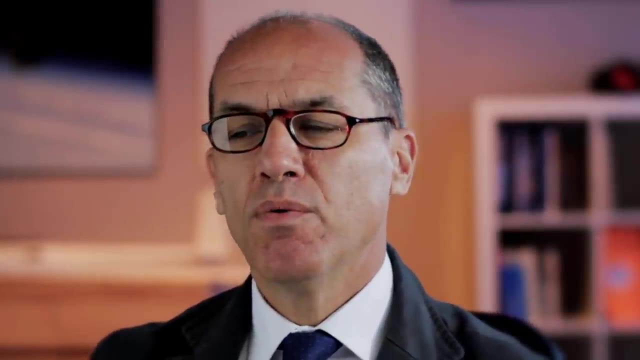 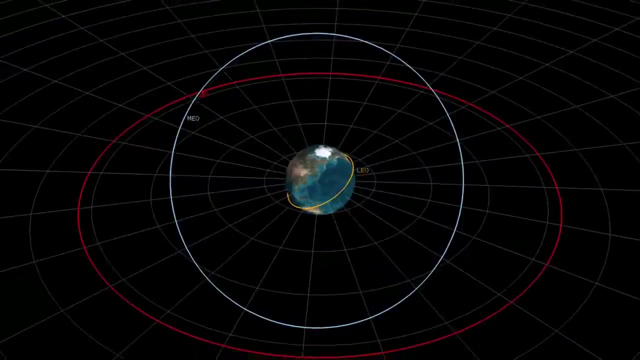 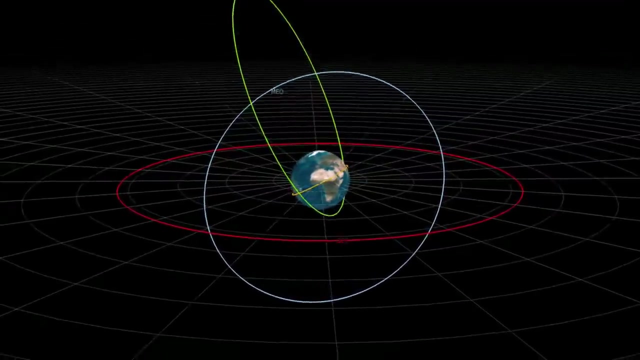 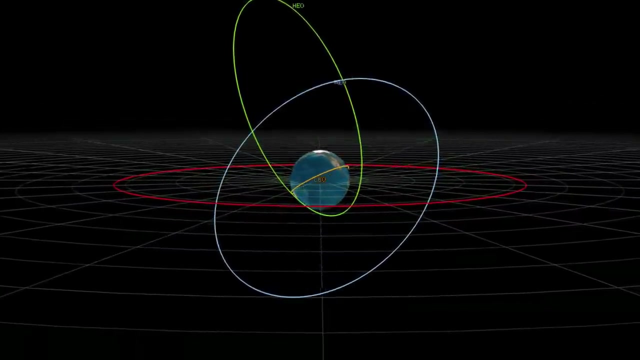 So we might enter now the topic of orbits, meaning where do we place such satellites and for which purposes. Of course, when we are talking about orbits, we think about something that's around Earth, while we can think especially for exploration or science, to go beyond the Earth orbit and to visit other planets or other natural 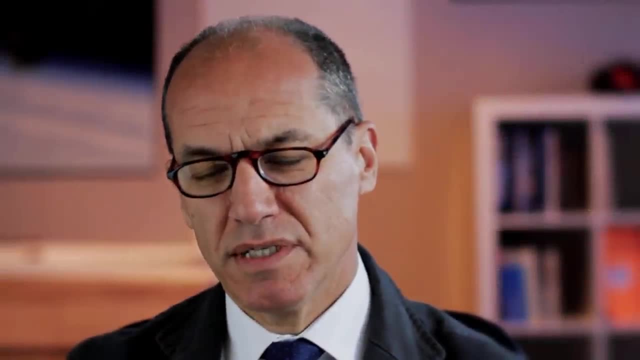 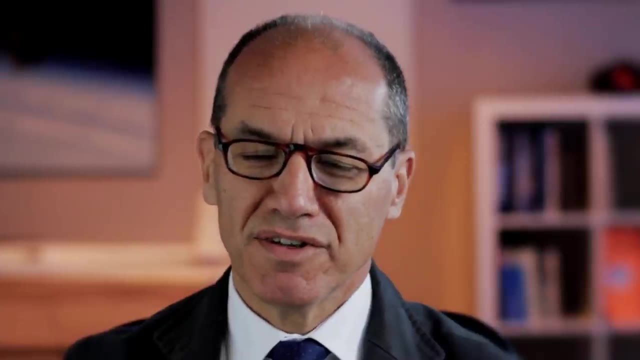 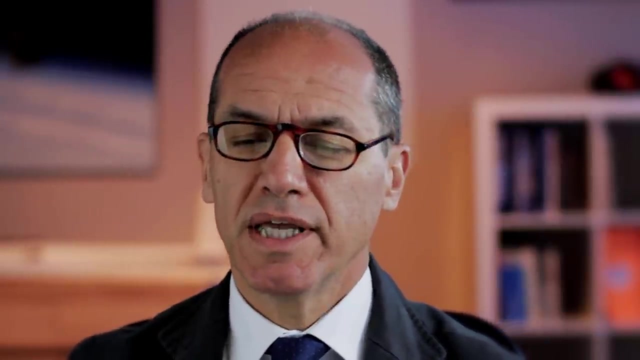 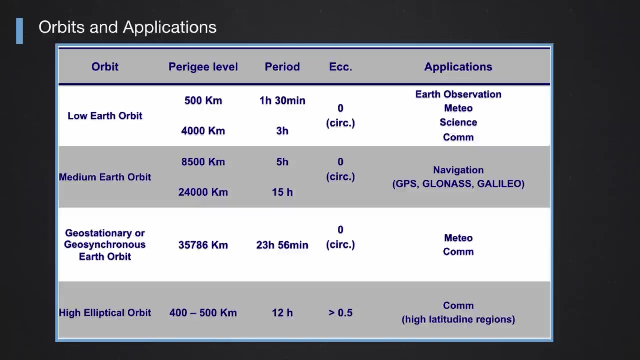 satellites or even going beyond our solar system. So there are a lot of missions that have trajectories or motion that are really very far away from our Earth. But when we are talking about applications, we might concentrate on orbits. Maybe the most important kind of orbit is the geostationary orbit, In this case the 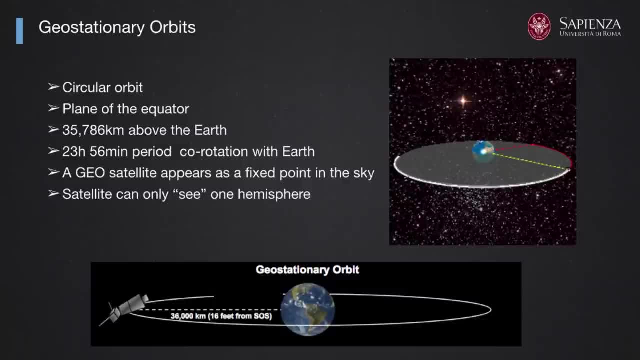 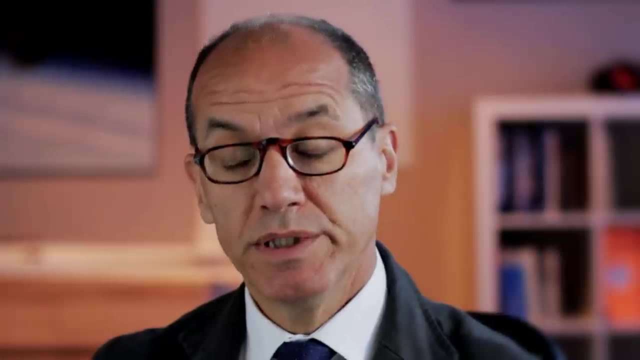 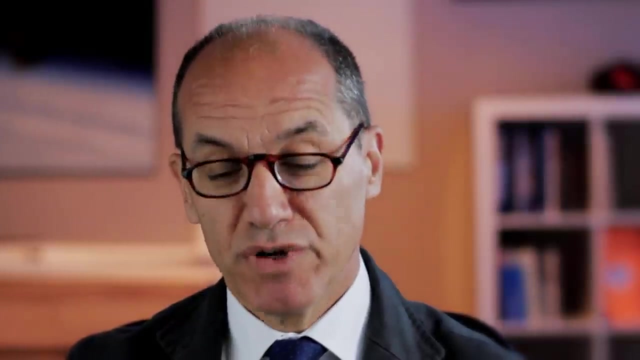 satellite is going on a circular path in the plane of the equator and the radius of this motion, of this trajectory, of this orbit, is around 36,000 kilometers. That means that the satellite is far away six times from the ground in terms of the radius of. 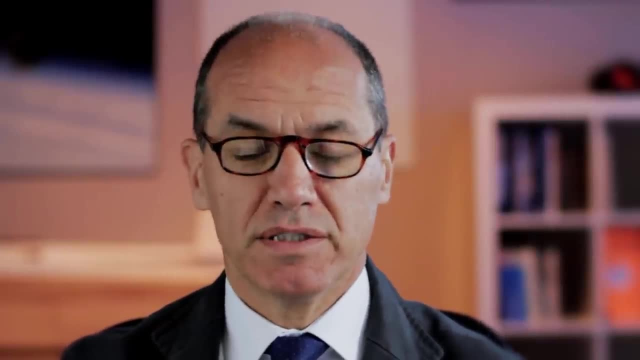 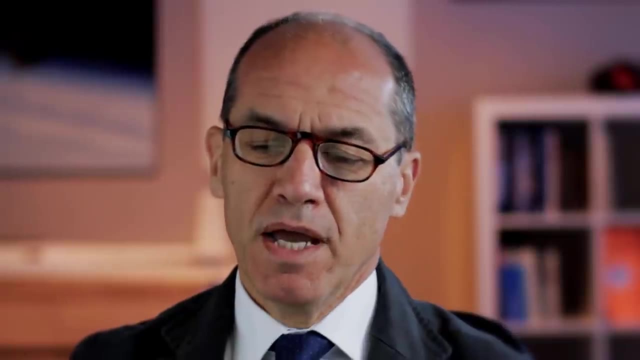 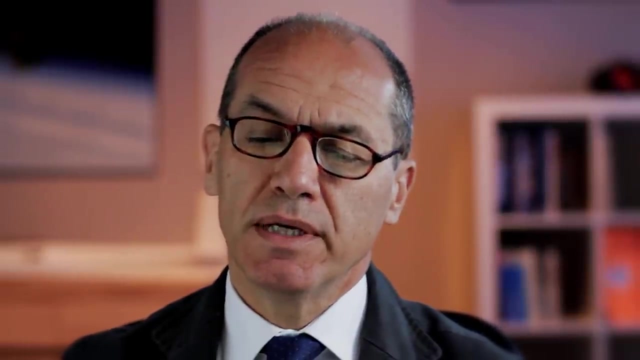 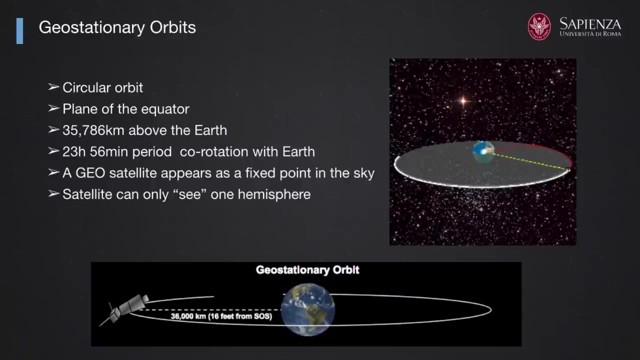 Earth. that is approximately 6,000 kilometers. So such satellites are very far away from ground. Why placing satellites in such an orbit? Because the motion of a satellite on an orbit is related to its velocity, So the satellite, to be stable on an orbit, should have a certain velocity by. 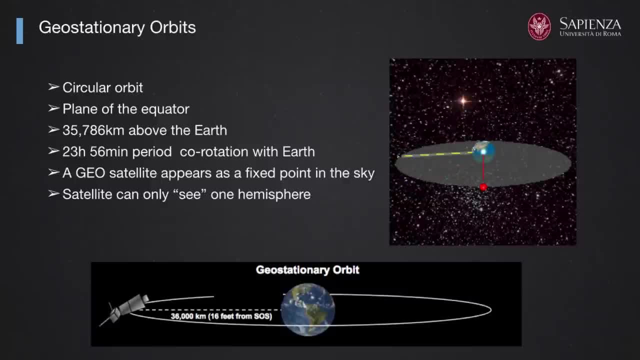 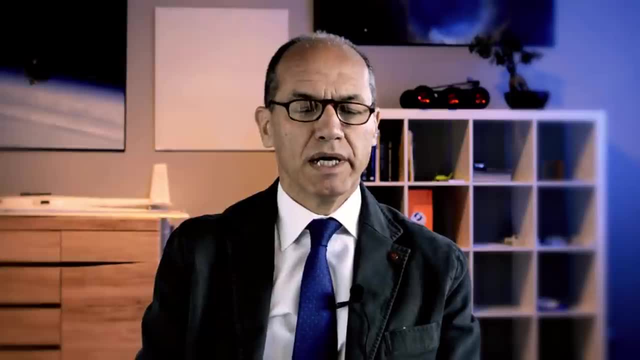 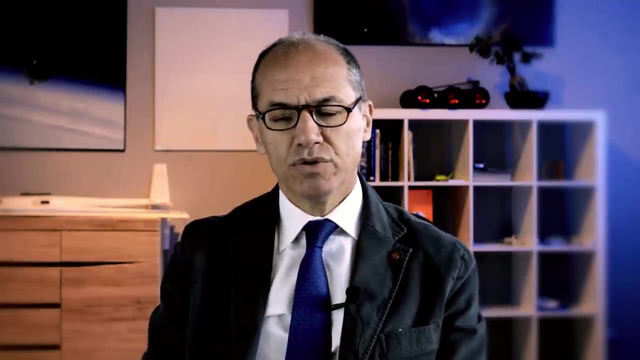 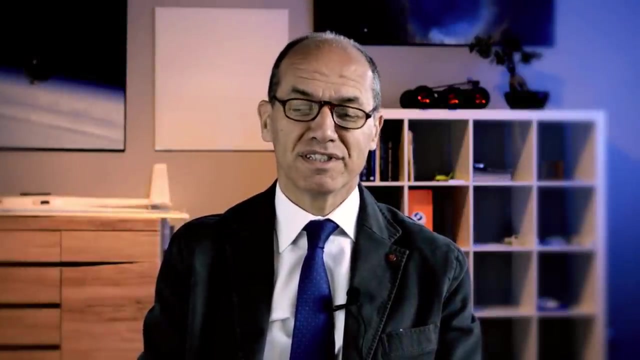 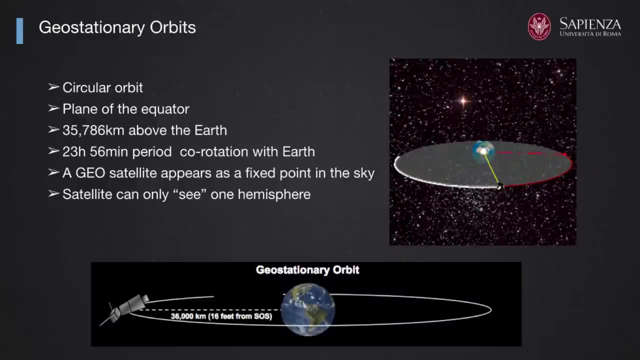 means of which, in terms of inertia forces produced by this velocity, the satellite is able to balance the force of attraction due to gravity. So, for that level of orbit, at 36,000 kilometers from Earth, the velocity of satellites in terms of angular 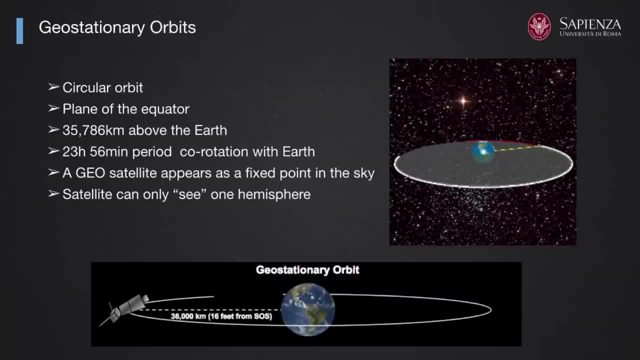 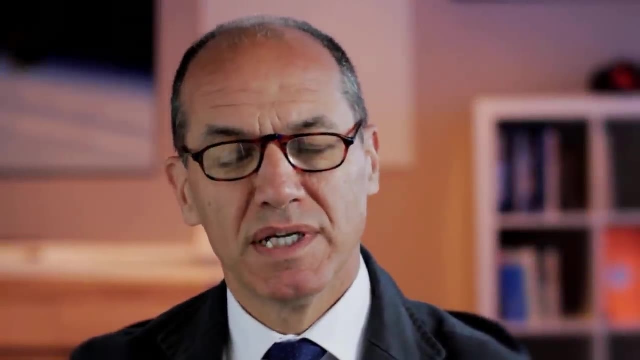 velocity corresponds exactly to the velocity of the rotation of our Earth around its axis. This means that in a geostationary orbit one satellite takes more or less one day to do a complete round. And since also the Earth is doing one round in one day, from Earth, 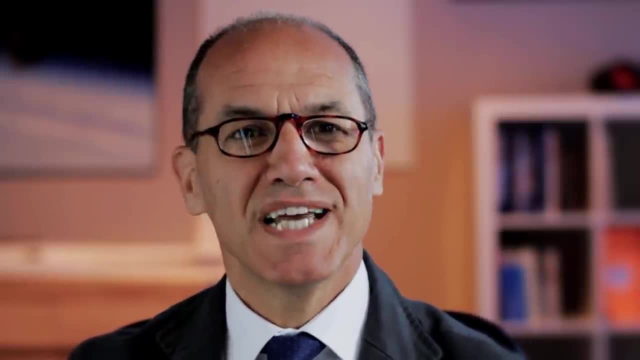 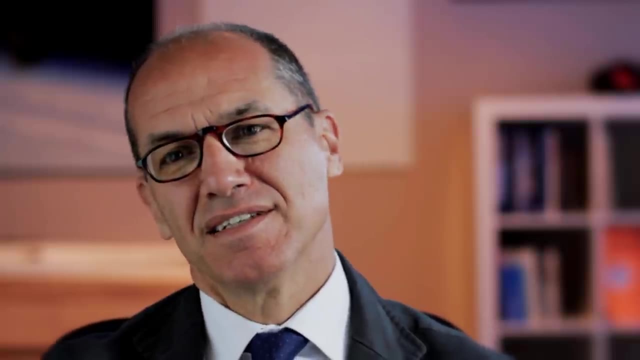 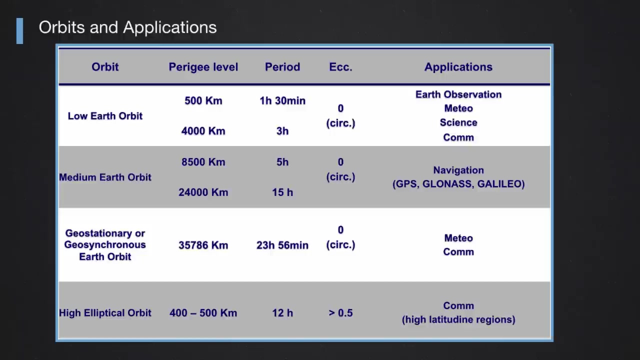 we see that this satellite is fixed on the sky like being a fixed star. So, being a fixed point in the sky can be used for telecom applications, since we can transmit to the satellite a certain signal, for instance from a TV broadcasting station and then from the satellite. 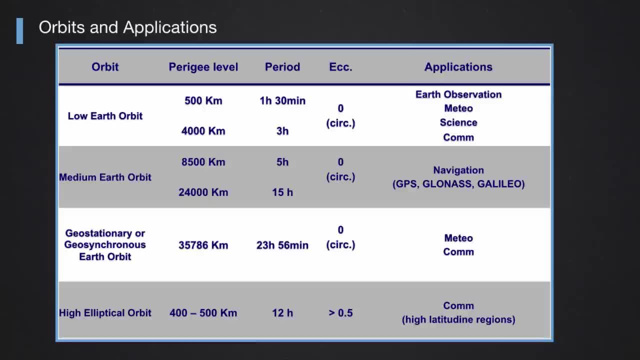 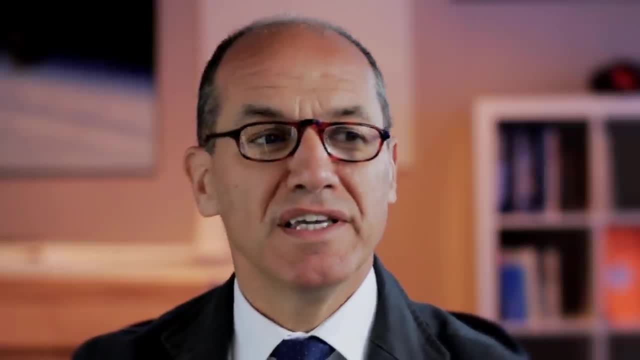 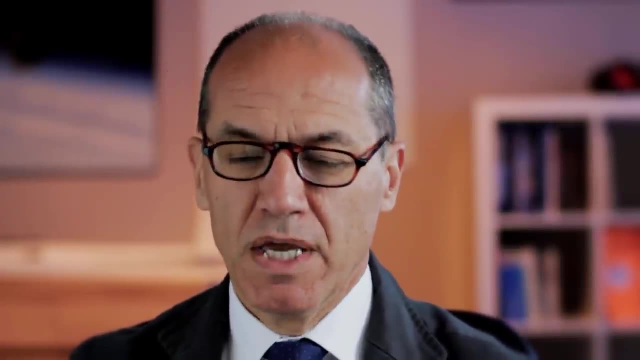 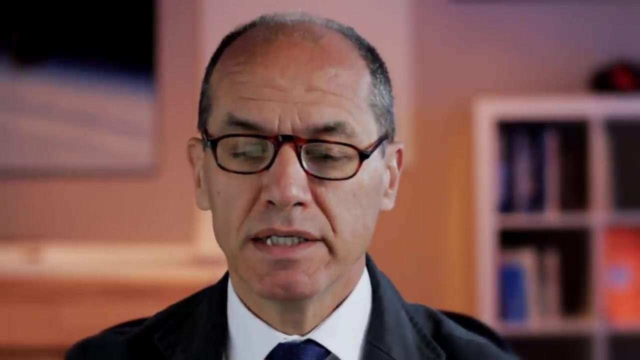 the signal can be provided in a very large area by means of the reflection of this signal and reach each and every house or each and every TV set on the area. So geostationary orbit is very, very important and there are positions on geostationary orbit that are being assigned. 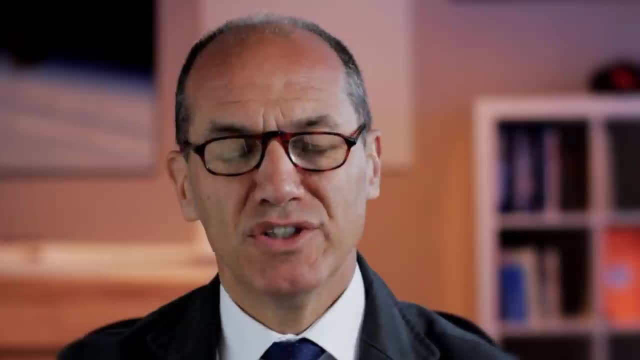 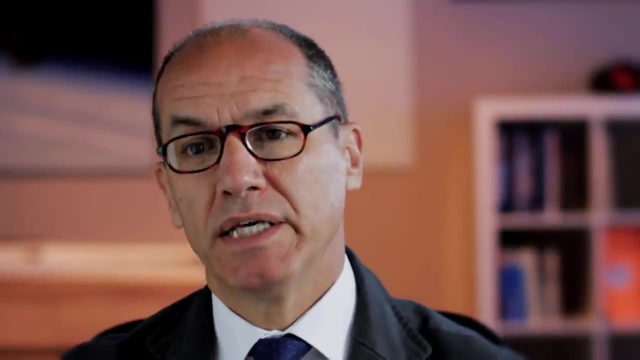 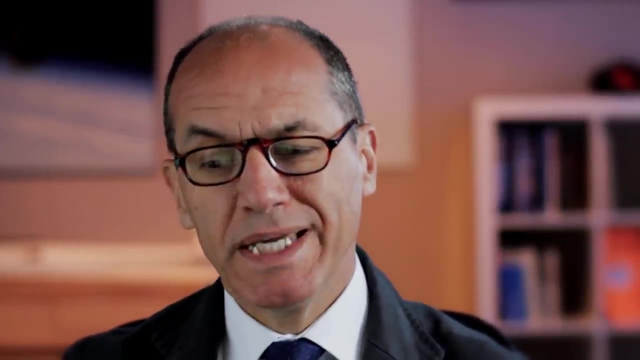 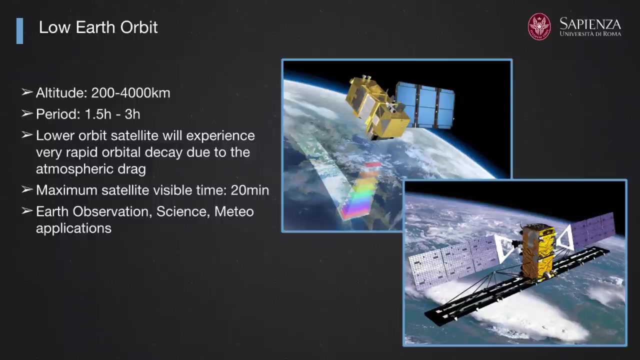 and basically all over the Earth. all around this circle, there are a huge number of satellites operating by providing telecom and especially TV broadcasting. But we have also applications in which other kind of orbits are used, and we call them low-hertz orbit. Low-hertz orbit. 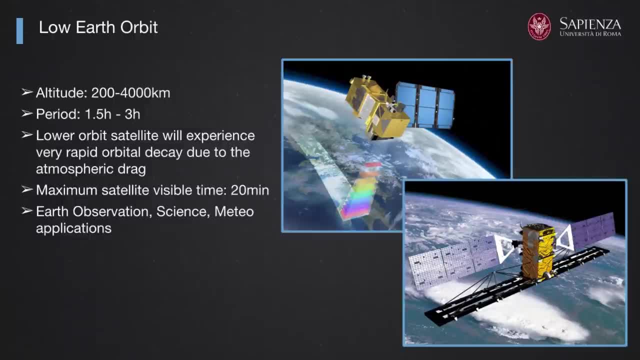 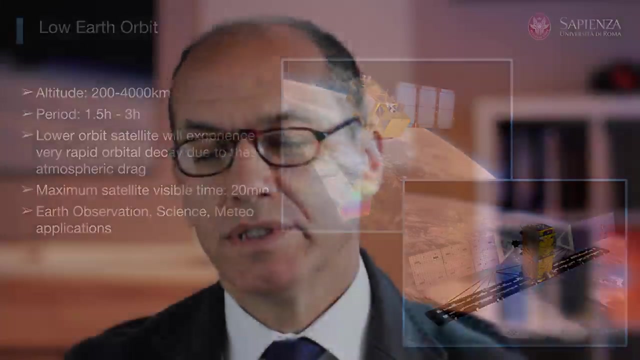 have a level between, let's say, around 400 kilometers up to maybe a few thousand kilometers, but the most of satellites are flying around 600-700 kilometers. In this case, the satellite is much closer to Earth and we use this kind of orbit. 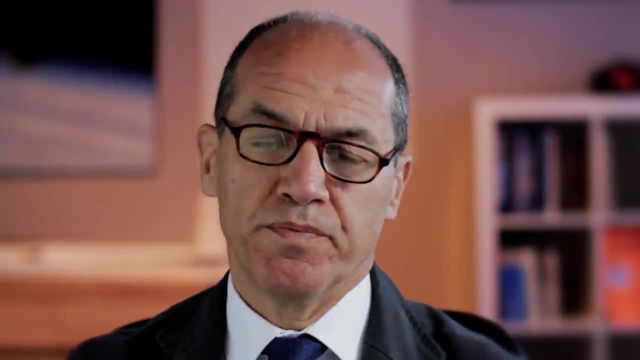 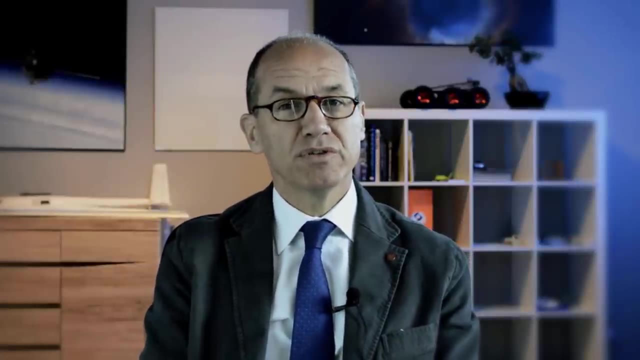 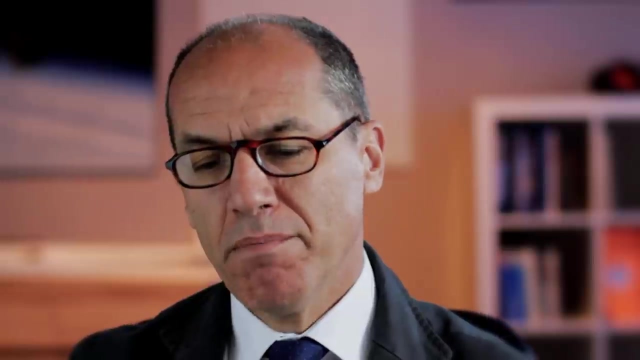 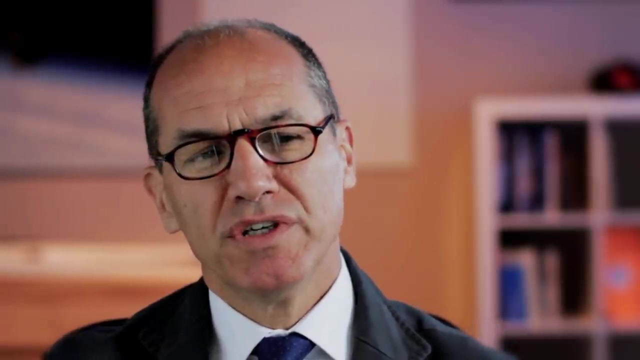 especially for doing Earth observation. Why this? Of course, if you like to make an observation of one thing, you like to be close and to see all the details. But there is a major advantage to go away from your target, because if you go away from the level of 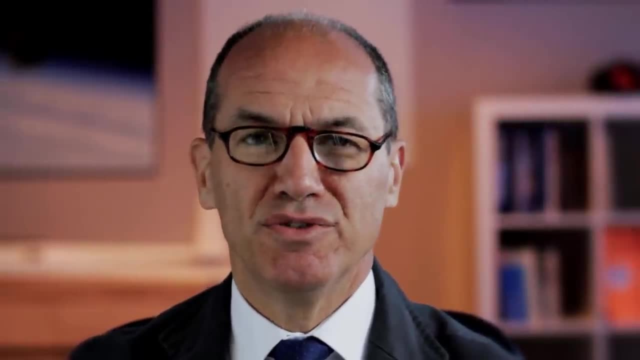 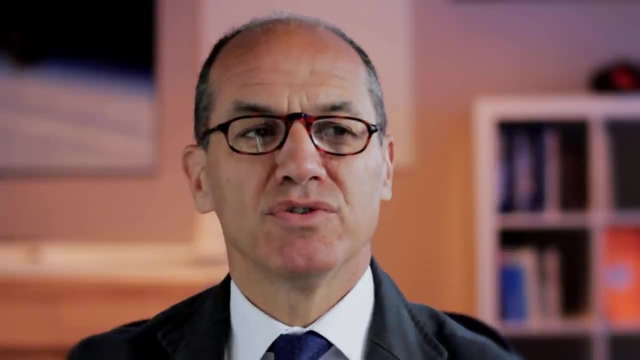 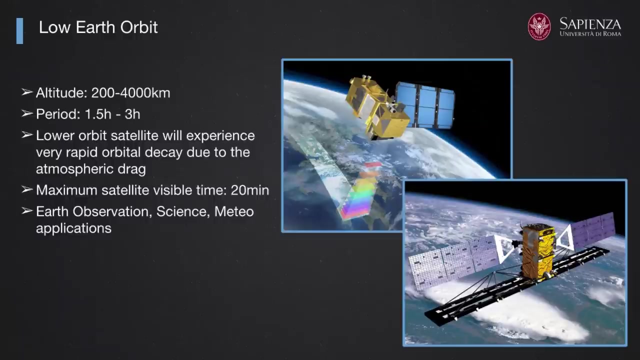 Earth. you widen your horizon, you see more things at the same time. So the idea is to go up and up, reaching those levels in order to have a much larger portion of the Earth that could be seen from the satellite. Then you place on board the satellite some payload, like a camera. 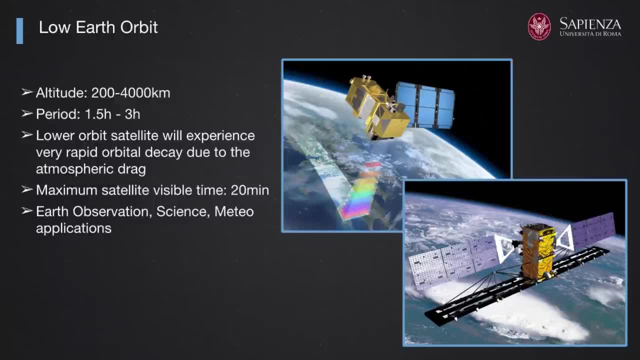 based on classical optical technology, or even you can place a radar, so another kind of sensor, in order to detect some information about what's on the ground. So what is done is to do remote observation And by doing that, by staying at this level, you can have: 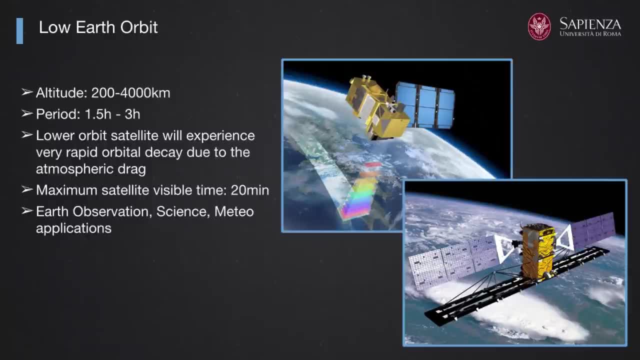 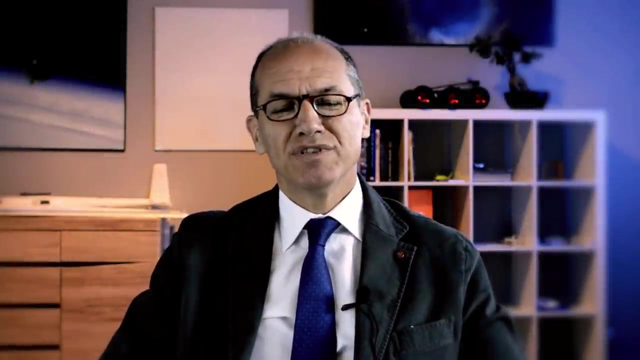 access to many, many places around the Earth. Why the orbit is placed at such an amount of kilometers, Why we are not going a little bit lower, like, let's say, 50 kilometers or 100 kilometers? because at that level the atmosphere is still there, and so the satellite is not capable of. working for long times because there is some friction with the atmosphere. so the energy that is related to the motion of satellite will be somehow damped by the interaction with the air and in very short time the satellite will diminish its level and eventually re-entering in the atmosphere and being destroyed. At that level, the velocity of the satellite will be much higher than the one of geostationary orbits, and so, instead of taking one entire day to do the complete round, the complete round will be done in a much shorter time, like, for instance, at around 500 kilometers in one hour and a half. So 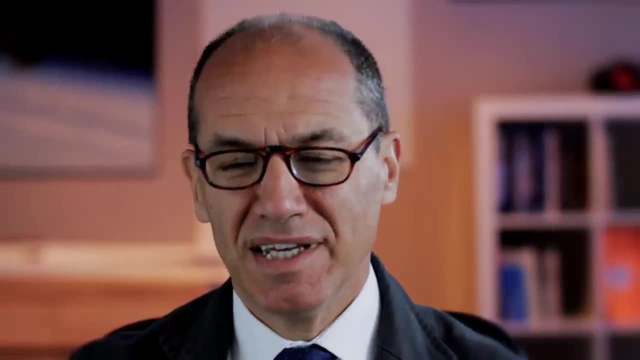 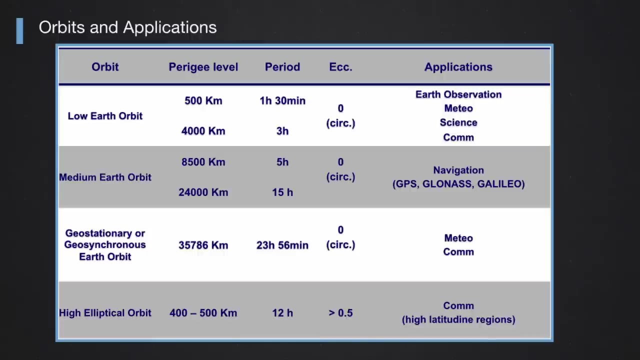 in one day there will be many rounds of the satellite on its orbit, With this low Earth orbit that are especially related to Earth observation. but of course you can do a lot of science application and some also meteo application. meteorological applications are typically run in 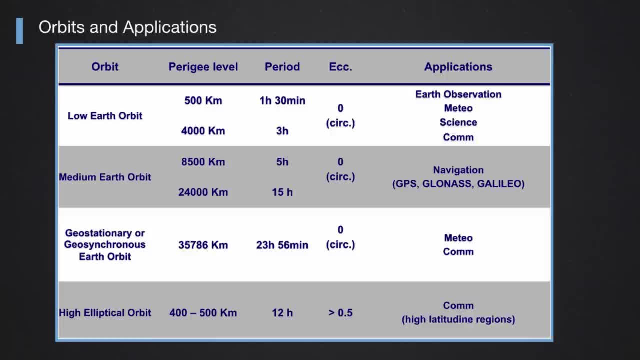 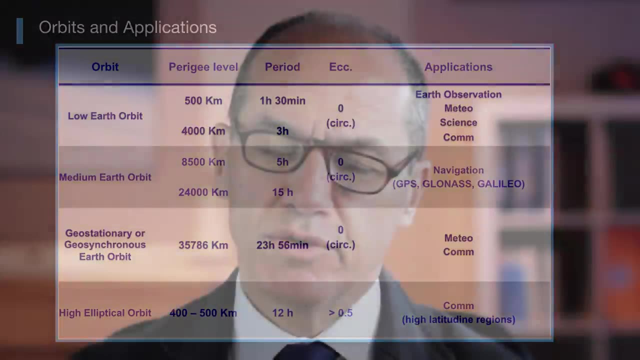 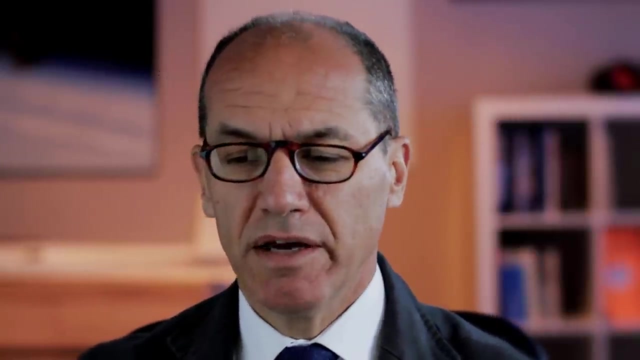 geostationary orbit for looking at the much wider area of the horizon. But one idea is to have the plane of those orbits in such a way that the rotation axis of the Earth is included in this plane. By doing that you might have this circular orbit of. 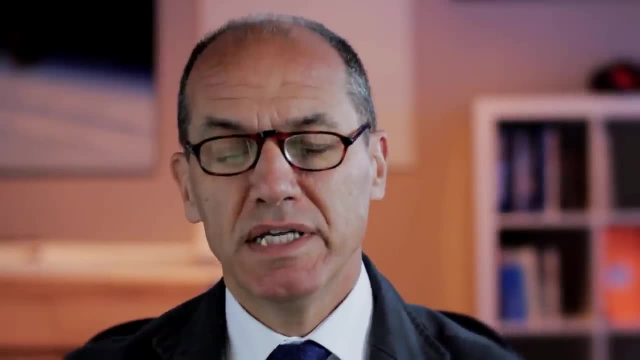 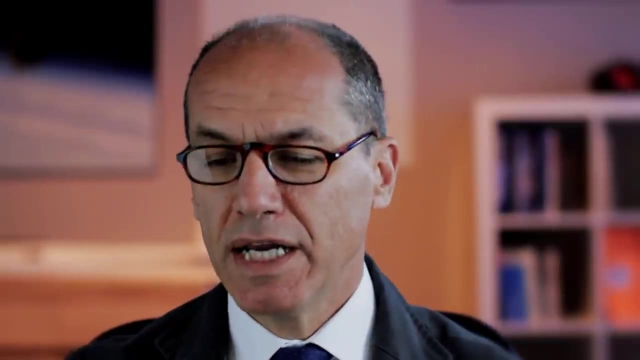 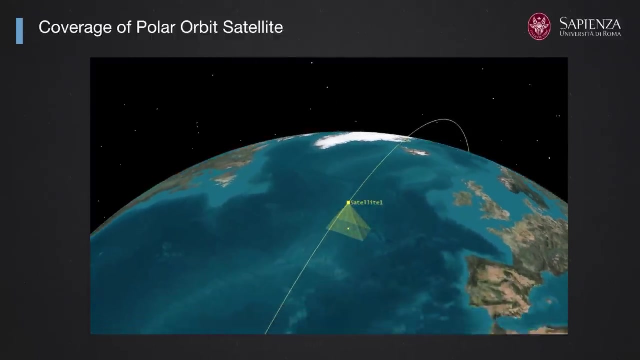 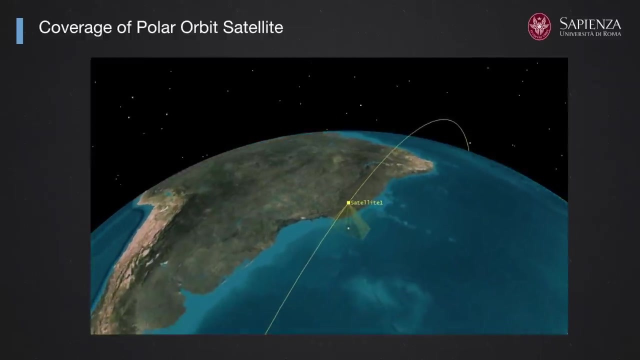 your satellites while the Earth is rotating below you, so the satellite will pass through different positions on Earth while the evolution of its orbit is going on, And this is a classical polar orbit or a synchronous orbit. by means, Earth observation applications are optimized in such a way that you can see. 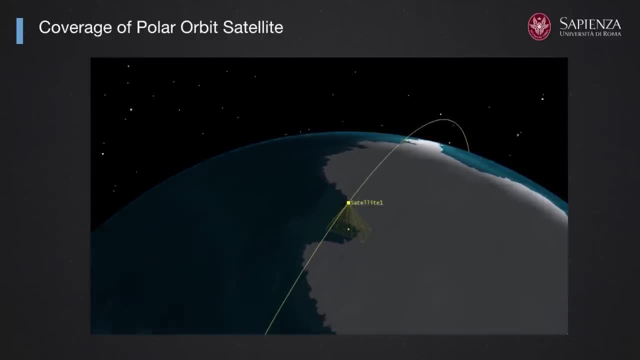 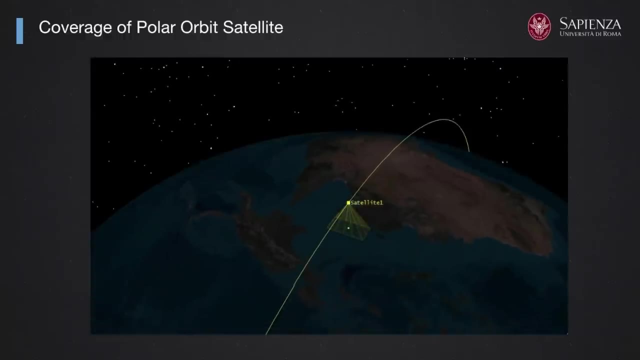 in a few hours, or maybe in one day, all the ground of the Earth passing below you, so that you can take pictures of all, of each and every place, on each and every spot on the surface of the Earth. So geostationary orbits and low Earth orbits. 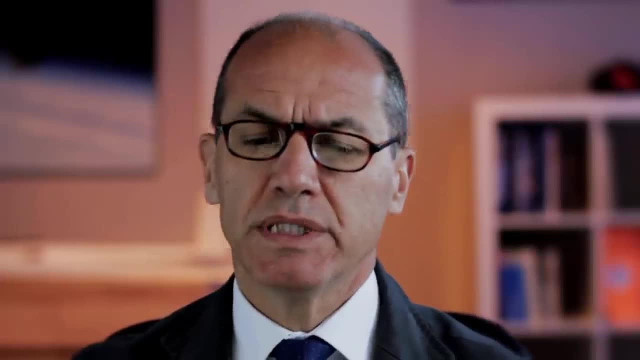 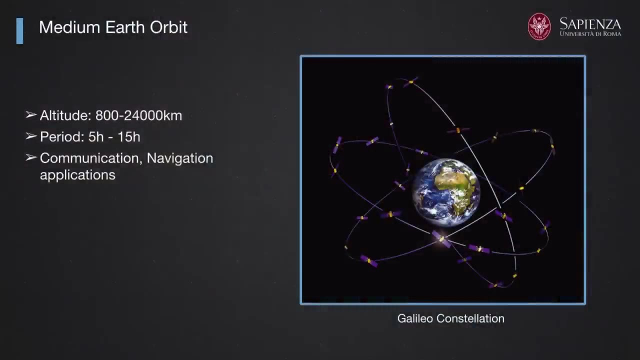 are very important. You have also other kinds of orbits, like medium Earth orbit. that are the ones used by navigation satellites like GPS or the forthcoming Galileo, or the Russian system GLONASS, And in that case you are in a 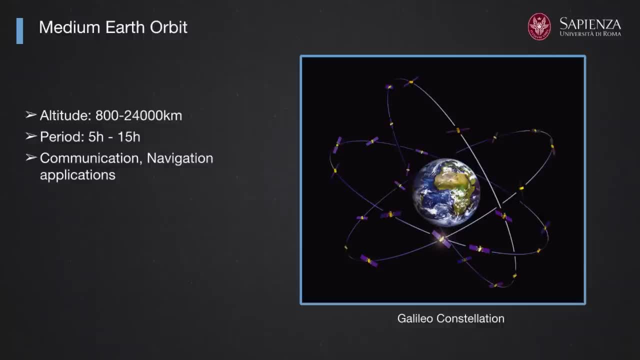 middle level between low Earth orbit and geostationary orbits, and you are flying around something like 20,000 kilometers In a circular orbit. In this case, for these applications you need constellations of satellites, not just one satellite is enough, and those navigation.